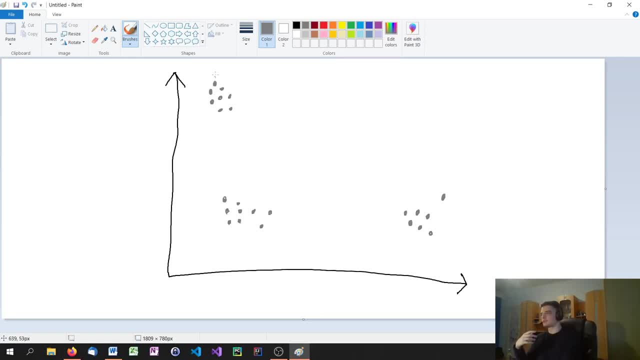 we don't have any classes, We don't say that this group of points here is red or blue or anything like that, or overweight, underweight or cat, dog or anything like that. We just say these are the points, all of them, and I 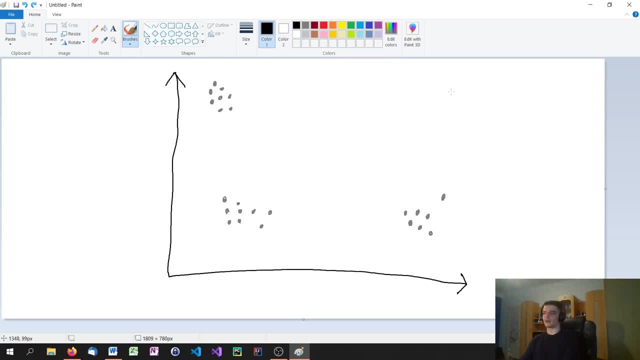 want you to find a certain amount- k amount- of clusters. so the algorithm that we're using here is the k means clustering algorithm and it's unsupervised. so we don't say: okay, here you have the red points, you have the blue points, you have the green points. now figure out what this new point. 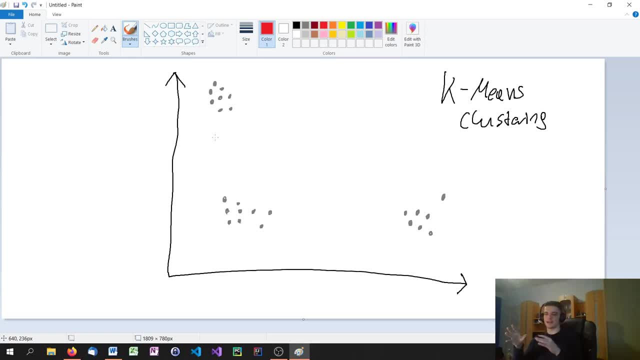 is. but we say, okay, just train the model on the data you have, find the clusters, find k amount of clusters and then basically, when a new point comes into the model or we get a new unclustered, if you want point, you can assign a cluster to it. so, as a human, we would see immediately, or as 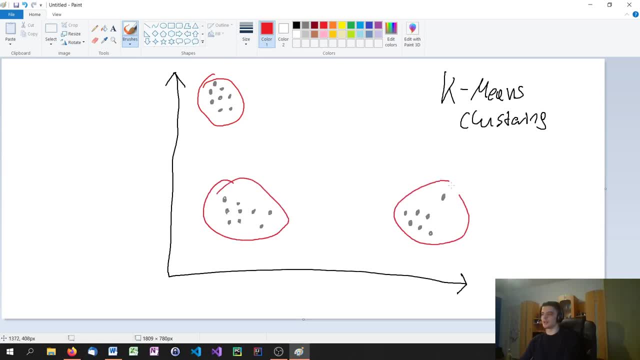 humans, we see immediately that this is one cluster. this is one cluster, and this is one cluster at least if k is three. so if we look for three clusters, these are the clusters. if we look for two, maybe we could say: this is one, okay, this is not. 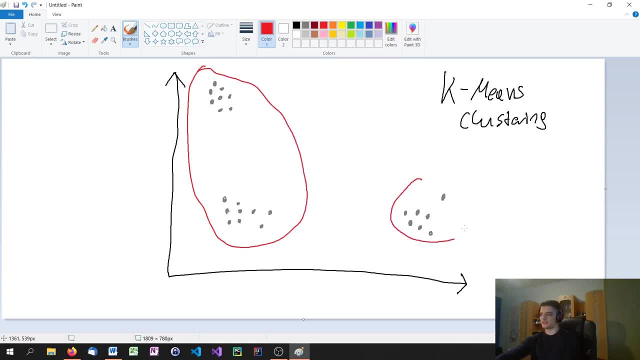 one, this here is one and this here is one. but, however, first of all, the data in real life is not as easy to cluster, because it's not that clear as in this trivial example here, and also we're not dealing with two-dimensional data only, but with 20-dimensional, 40-dimensional data, because 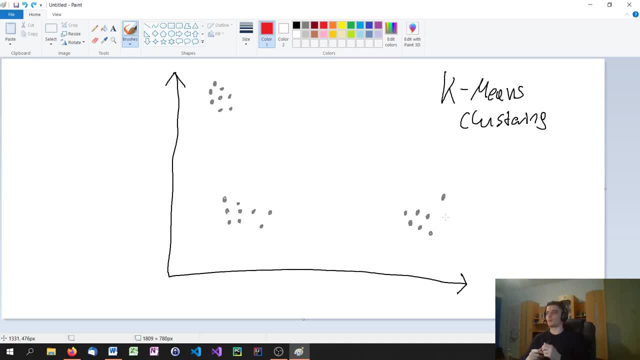 we have a lot of different features and also we need to train an algorithm to do that. we cannot just say to the computer: figure out the clusters here, because the computer does not work like a human, it does not work like a human. it does not work like a human. it does not work like a human. 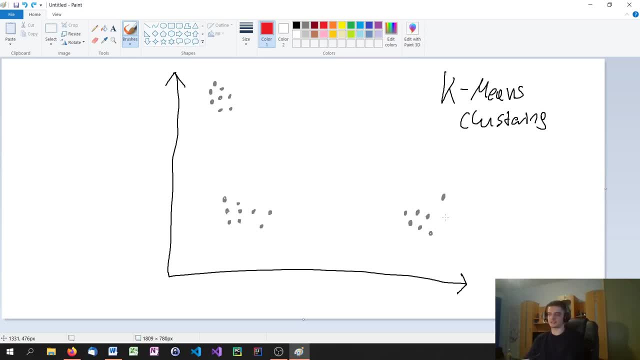 you cannot just say: okay, i see the patterns here, so this is a cluster, this is a cluster. a computer needs an algorithm. so what we're going to do here is we're going to define k being three. so let me just write that down here: k equals three. and we're now going to say, okay, we 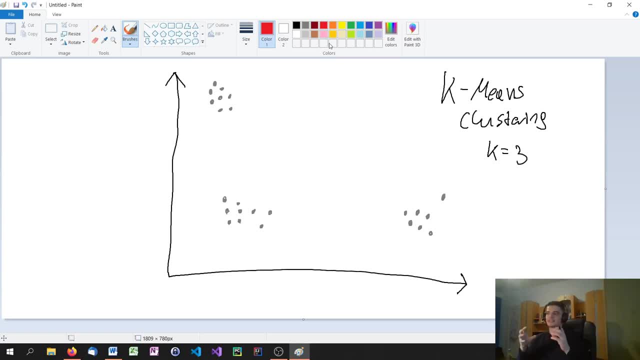 start with three random centroids, and the centroids are basically the center of, or the centers of the cluster. so let's say we have this red triangle here, which is the centroid of the cluster red, then we have the green one here. actually, let's pick dark green, dark green. it's better for the 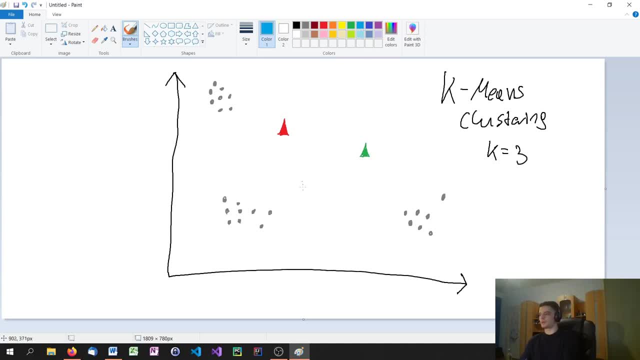 video, i think, and then we have a blue one, i don't know, maybe somewhat like that's a little bit tricky right now. uh, let's say we have one here to make it a little bit more interesting. however, these points are, or these centroids are, basically random, so we don't choose them, we don't place. 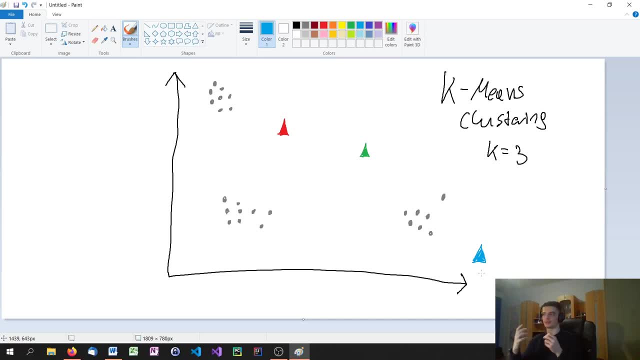 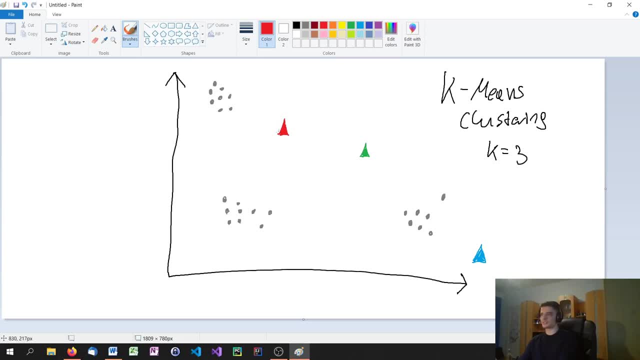 we're going to say, okay, the red one is the nearest one, obviously, because, uh, as you can see, there's the green one is way far, way more far away, and the blue one as well. so we're going to say, okay, these are now the red data points. they belong to the cluster red. 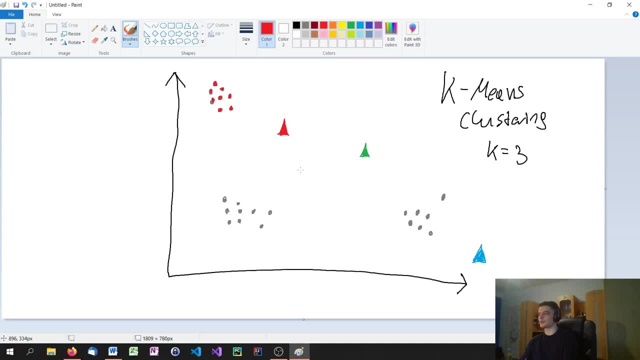 because obviously they are. this is the nearest centroid, um, then we have these here at the bottom, and here it's a little bit tricky. we could say, for example, that this is a red one, maybe, um, and maybe this is a red one, but the rest might be more of a green one actually. 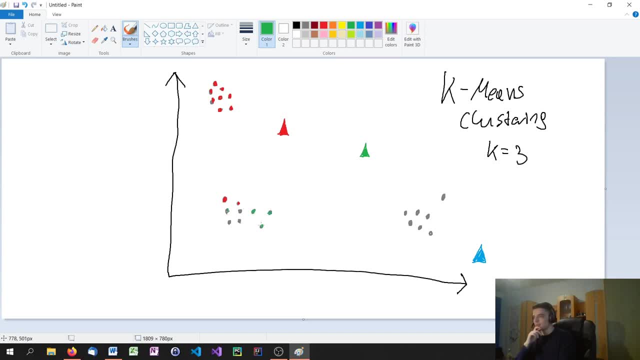 maybe it's not that accurate what i'm saying right now, but it's just an example. the algorithm will do this with accuracy. it will. it will just measure the distance between the centroids and the individual points and then figure out which centroid is the nearest to which point. so we always have to calculate this, and then we also have some of 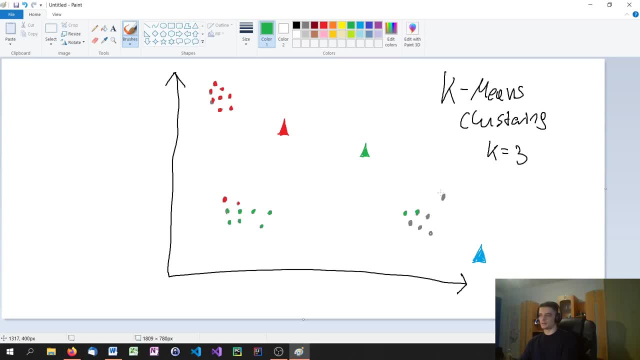 these here. let's say: this is green, this is green, uh, let's say, this one is green as well and the rest is blue. so these would right now be our uh clusters. so we would say these four points: here are the blue, uh, the blue cluster, the green ones are the green cluster and the red ones are the red cluster. now, of course, this is not 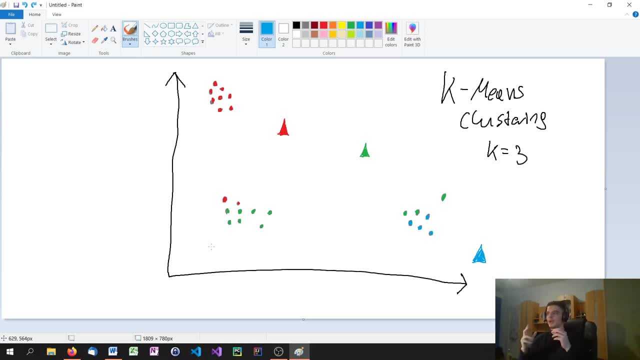 accurate right now, so we need to make an iteration here. what we're going to do now is we're going to pick the centroids and place them in the center of all these points. so what we're doing here basically is we're deleting the centroid that we already have and we're taking a new centroid, or 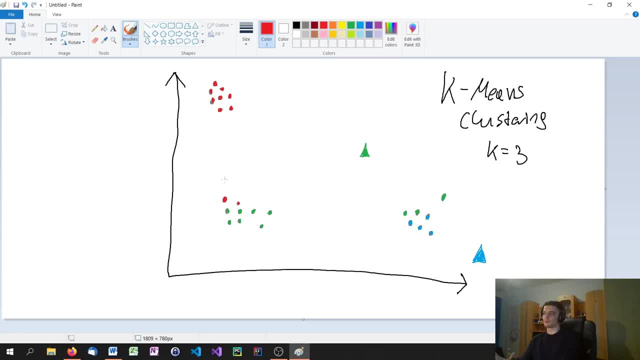 creating a new centroid, placing it in the middle of these points. so we have two points down here and a lot of points up here, so the centroid might be somewhere around, i don't know. let's say here: this is a reasonable centroid, a reasonable new centroid. uh, so the green one would be, uh, actually somewhere in the middle here, but more to the left. 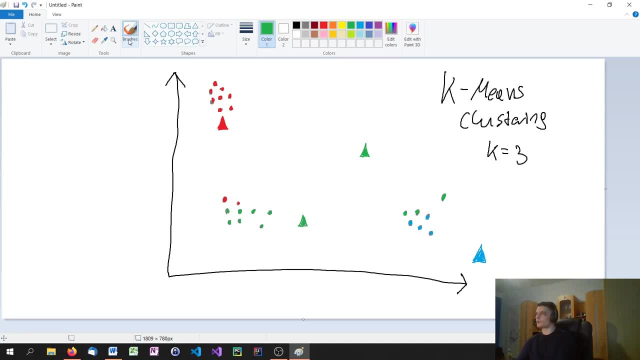 something like this one here and the blue one would just be right in the center here, because all the blue points are here and now. what we do is we are going to take a new centroid and add this point here and now. what we do is we are going to 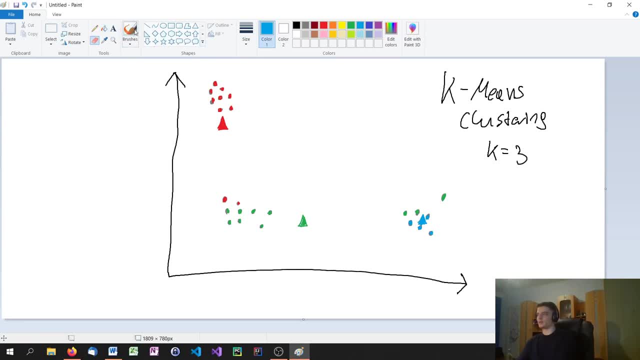 is, we do the same thing again. we ask ourselves now, with the new centroids, which points belong to which centroid? and of course the red ones stay the same. but these red ones here, these two red points down here, are actually green right now. so we're going to say, okay, green, green. 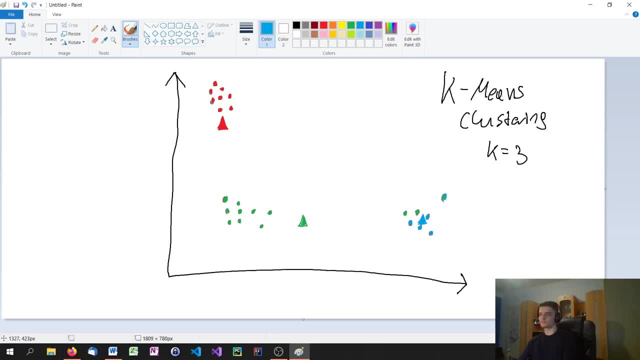 and all these points, of course, are blue. so now they are blue, and again we do the same thing. we adjust the centroids, we say okay, again, put the centroids in the center of all the points, and then we end up with the optimal centroid here in this case, which is right in the middle. 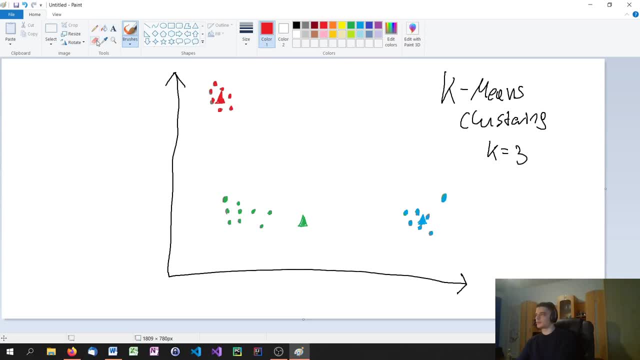 of all these points and the same thing is for green and for blue. so let's okay, blue is actually quite good and the green one would be right here in the center. so now we have the centroids and we stop when we notice that not a lot of things are changing anymore. 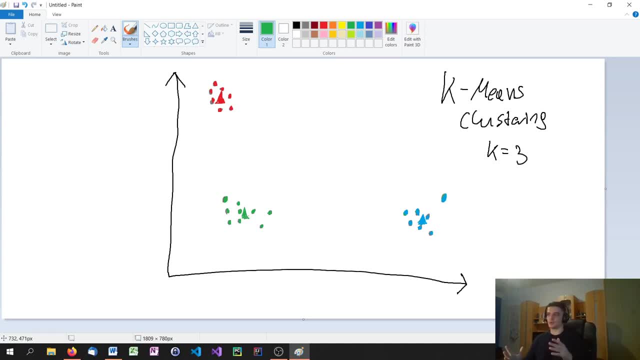 because right now we're not going to make any changes. the points are clustered well, so this is actually the optimal model, and this is what we always do. we adjust the centroids, adjust the point classifications or clusterings, then adjust the centroids again until there's not much to change anymore, and this is how k-means clustering basically works. so, in order to start, 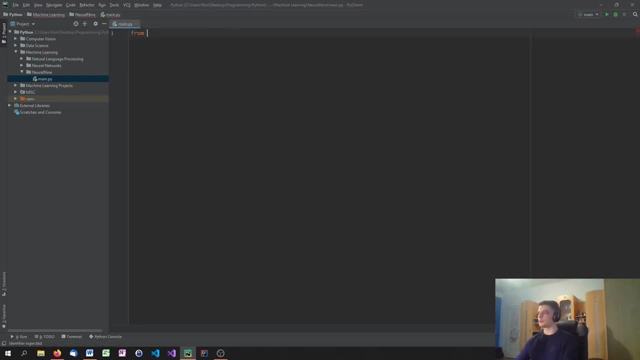 working with k-means classification in python, we need to import the respective modules, so from sglearncluster- import k-means and from sglearnpreprocessing import scale, which is the function that we're going to use to normalize the data. so basically scaling it down from zero to one and the data that we're going to use here is going to come. 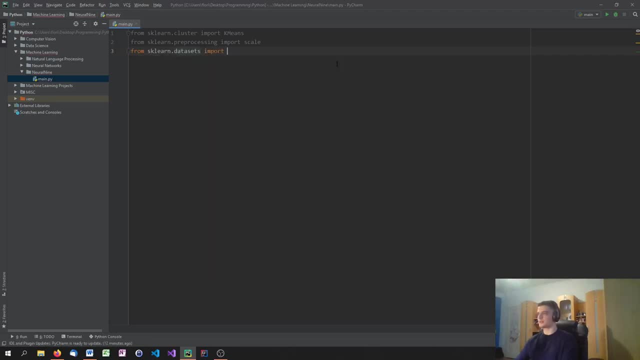 from sglearndatasets and the data is the digits dataset. so we're going to import load digits and the digits dataset is basically just a dataset of handwritten digits scanned into a computer. um, so we have the digits from zero to nine and we can classify them with. 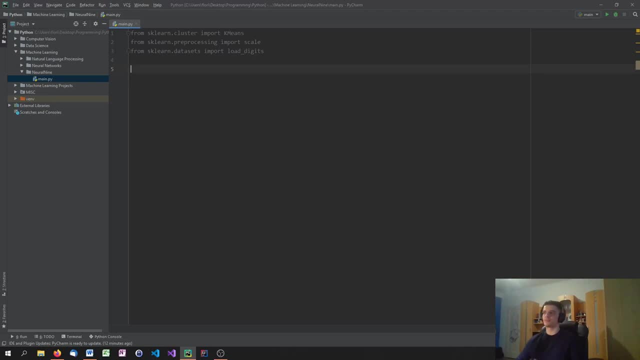 classification algorithms, but in this case we're just going to cluster them. so we have a bunch of pictures of ones and twos and threes and nines and sevens and all that, but in the end we're not going to say these are the sevens or these are the nines, and when we enter a new number we're 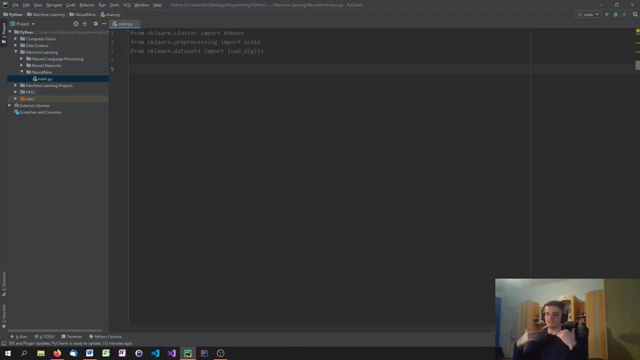 not going to get a result of: this is seven or this is six, but we're just defining clusters, so we're spotting the patterns in um, in these, uh, in the data, and basically then we're adding new data to it to see which category it fits in. so we're not telling the model which number is which class. 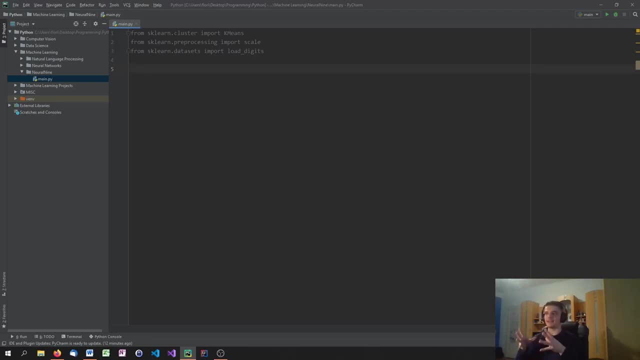 so we're not saying this is a nine or this is a seven. we're not making it that easy. we're just inputting a bunch of pixel and expecting the model to figure out itself which numbers are similar and which are not. so this is what we're actually doing, and 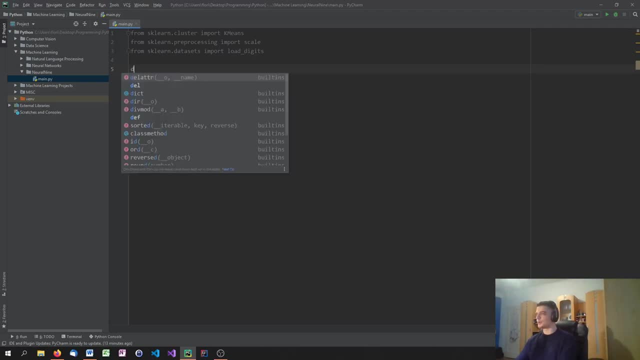 you. so for this we're just going to import or to load the digits. so we're going to say: digits equals- load digits. and then we're going to say data equals um. data equals scale dot digits. so this is the data right now. and in order to train the uh k-means model, we're just going to say: 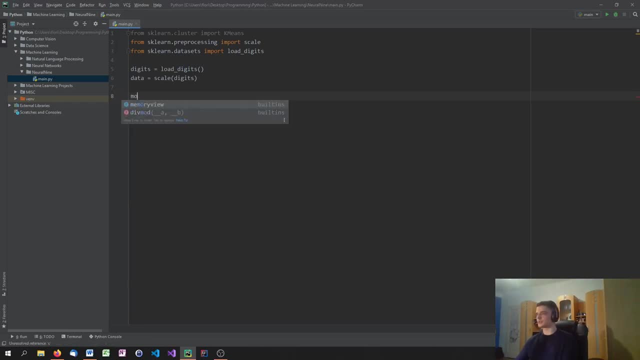 actually clf is not true here, because we're not classifying. let's say just model equals um, k-means, and here we have to specify a couple of things. so we're going to say that, we're going to say a couple of parameters, and the first one, of course, is how many clusters are we going to use and in? 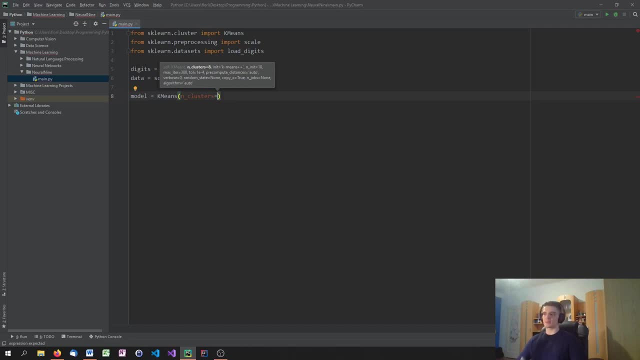 this case, uh, no number, but 10 makes sense because we have 10 different digits. so it doesn't make sense to use 20 or, uh, five different clusters because we have 10 digits and as soon as i try to look for a different number it's going to start doing some crazy shit because, of course, 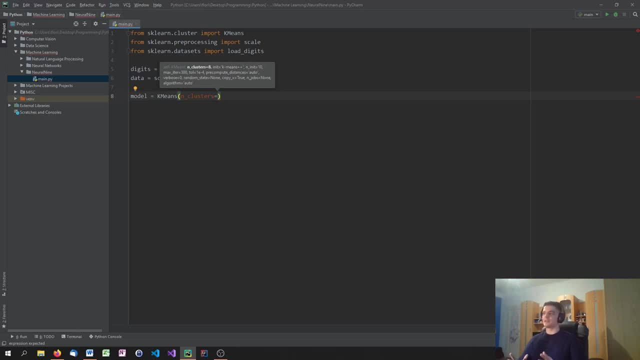 every eight looks similar, similar to every other eight. but if i look for two classes, for examples, uh, how would you? how would you separate these into two clusters? so how would you separate all these digits in two clusters based on the pixels? it doesn't make a lot of sense, so we're going to pick 10 and then we're going to pick an initialize. 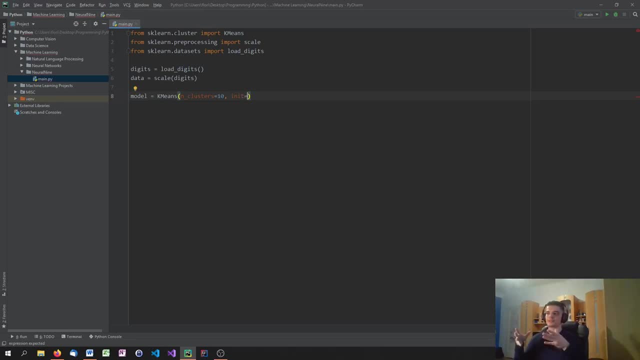 uh method, so some system of determining the starting point of the centroids. i'm just going to pick random here, so just random starting points, and we're also going to choose how many times it should start with different um initializations, so with different initial points for the centroids. 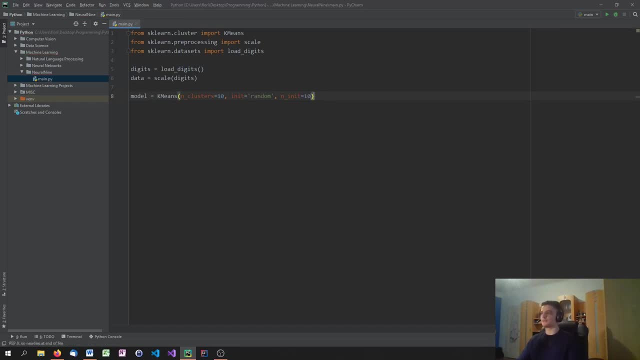 and in this case i'm just going to say 10. we want 10 different starts to see which one is the best. and finally we just have to say modelfit data and that's it. then we can train our model and we're not going to see a lot. actually, what the fuck is that? 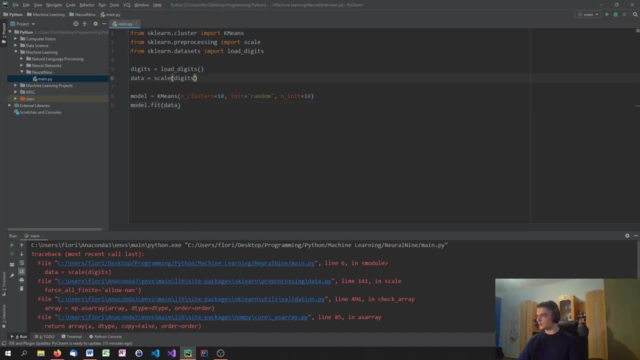 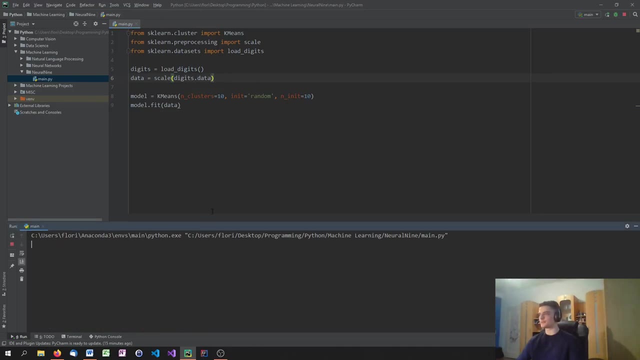 uh, scale digits, oh sorry, scale digits, dot data, of course, not digits itself, because we just want to scale the data of the digits and of course we don't see anything. the model just trains and that's it. and also, it does not make a lot of sense to test this, because we 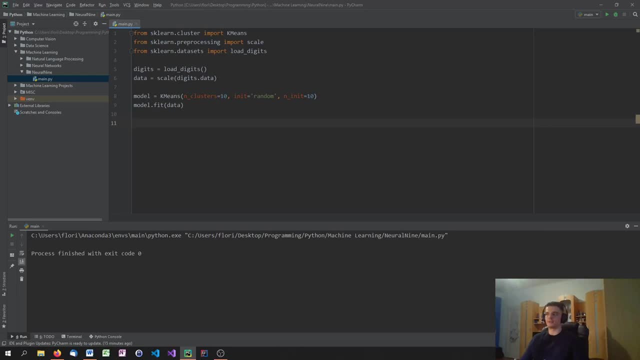 don't have a measure of true or false. this is unsupervised learning. we don't have something to tell us. uh, is this a true clustering? is this a true classification? we just have some clusters and we can add new data and, of course, we can go ahead and say modelpredict and add new pixels. 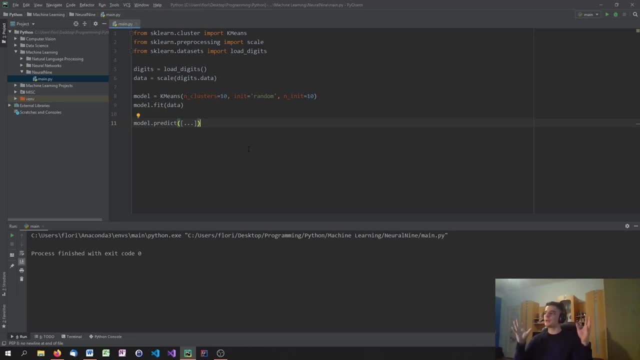 and we're going to talk about how to do this in a future video. but we could just read in a handwritten digit and classify it with this or actually not classified, sorry. add it to a cluster with this predict method here. so we would just add our picture and think about which or look at.